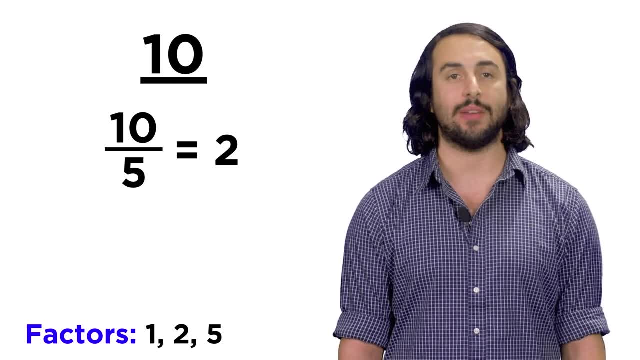 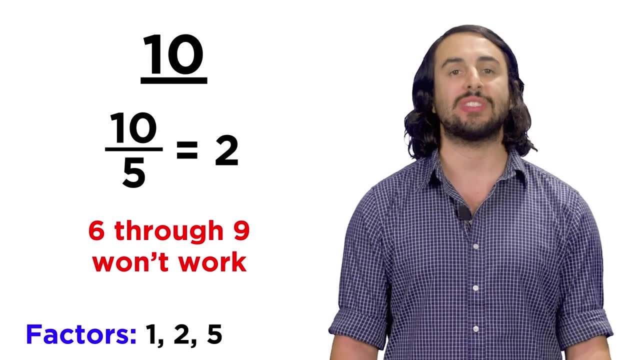 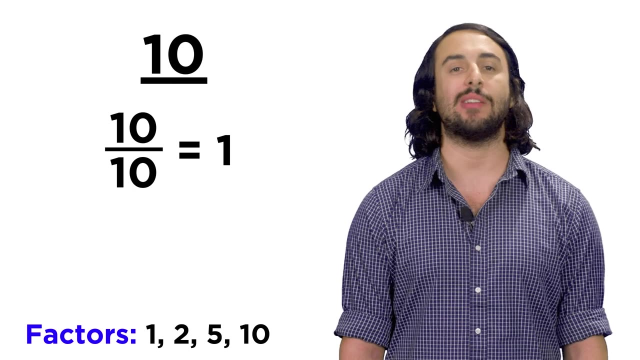 Ten divided by five is two, So five is a factor of ten. But from there no number bigger than half of the larger number will be a factor except the larger number itself. so six, seven, eight and nine are out. And lastly, we say that ten is a factor of ten because ten divided by ten is one. 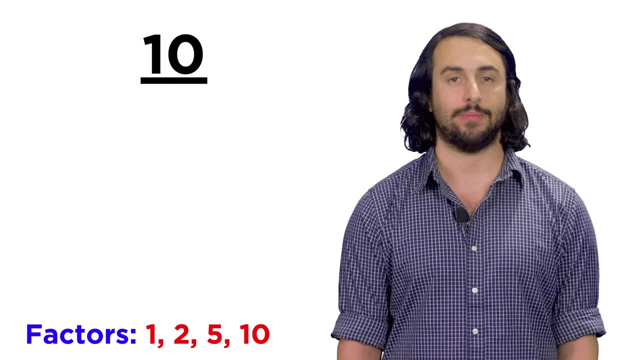 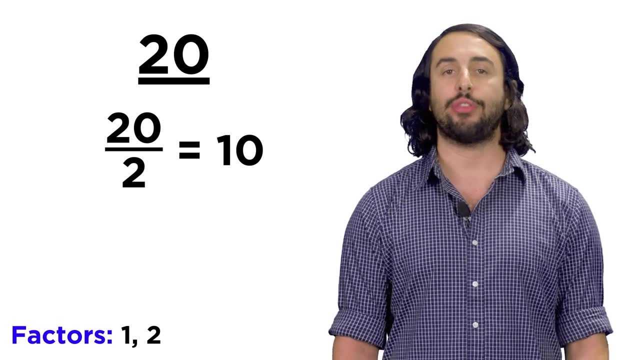 One, two, five and ten are the factors of ten. How about twenty For twenty? we see that one works, One works as always, Two as well, because it's an even number. Three does not, but four does as well as five. 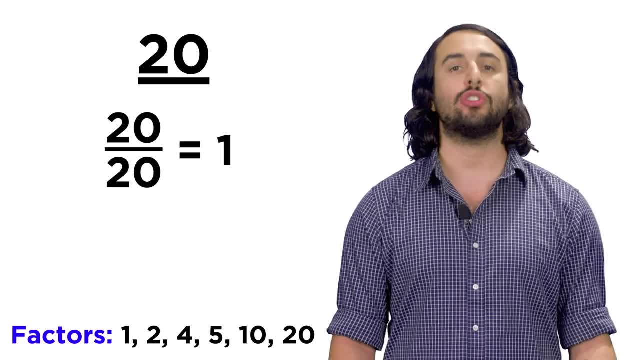 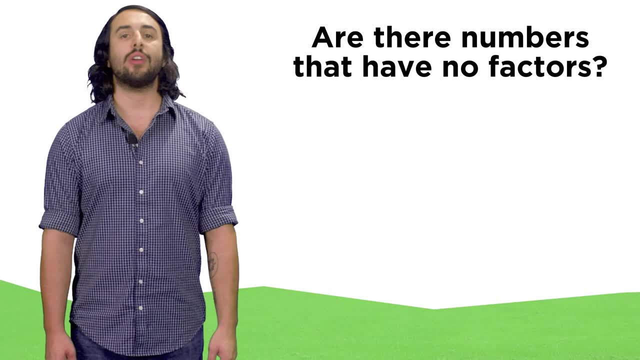 Then we jump all the way to ten, since it's half of twenty, Then twenty itself, and that's the end. Those are the factors of twenty. This brings us to an obvious question: Are there any numbers that have no factors whatsoever? 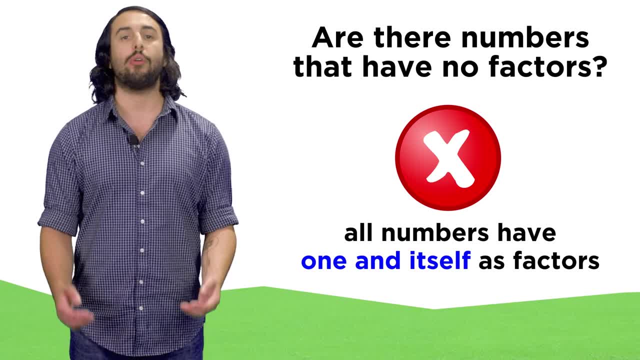 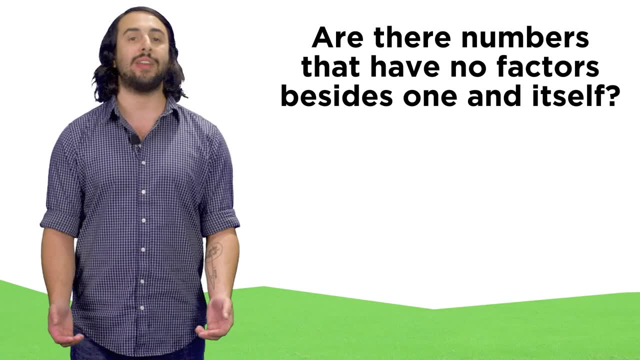 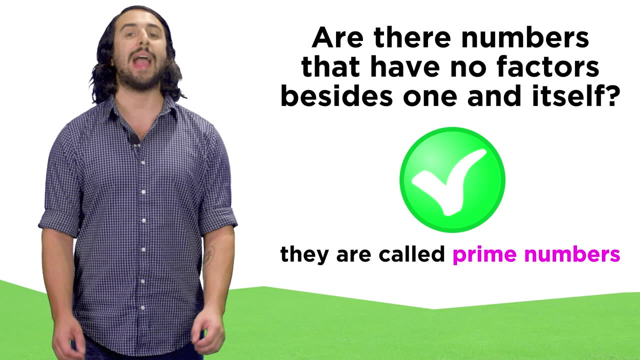 Technically no, because any number will have as factors both one and itself. But what about beyond that? Are there any numbers that have no factors besides one and itself? There are indeed many, and numbers that fulfill this criterion are called prime numbers. 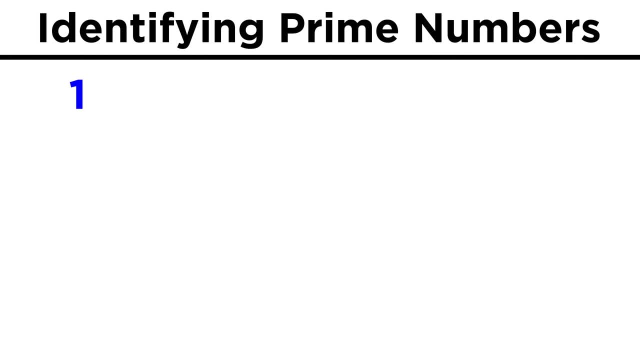 What are the prime numbers? One doesn't count, because one and itself would be the same thing. So let's start with two. Two counts, as does three, because these are so small that there can be no other factors. But once we get to four, four is divisible by two. 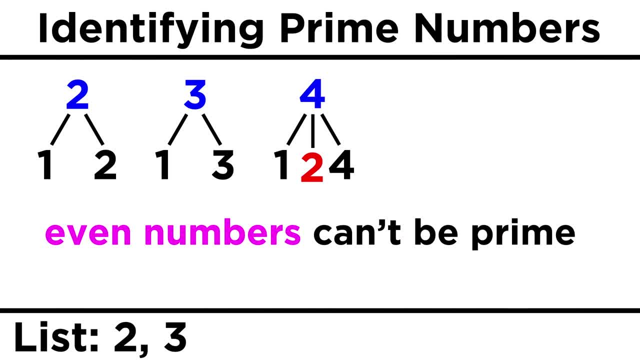 So four is not a prime number. In fact, no even numbers, except for two, can be prime numbers, because they are all divisible by two. Only odd numbers can be prime numbers. Five is a prime number, as is seven, but nine is not, because it is divisible by three. 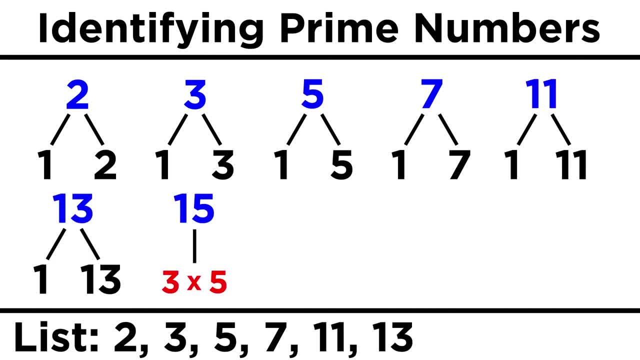 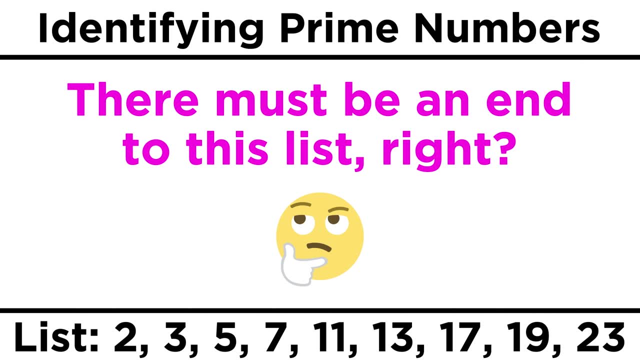 Eleven works, as does thirteen, but not fifteen, since that's the product of three and five. Seventeen works, and so does nineteen, but not twenty-one, since that's seven times three. Twenty-three works, and so on. One would think that this can't go very far, because once numbers get big enough, 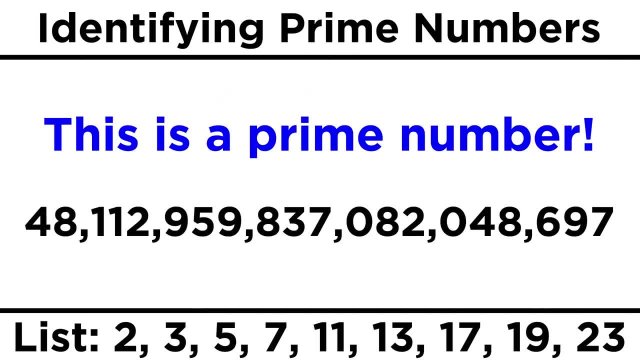 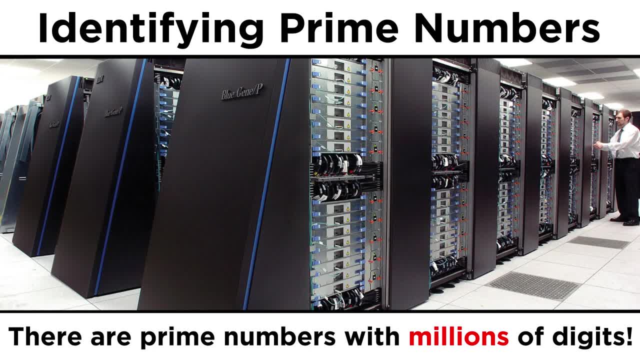 there have to be some factors in there, But there are some astoundingly huge prime numbers. The largest one discovered so far has millions of digits, which is mind-boggling, and it took thousands of computers running simultaneously for days to find this number. 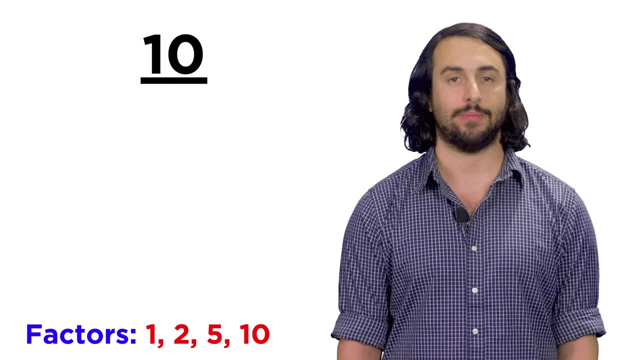 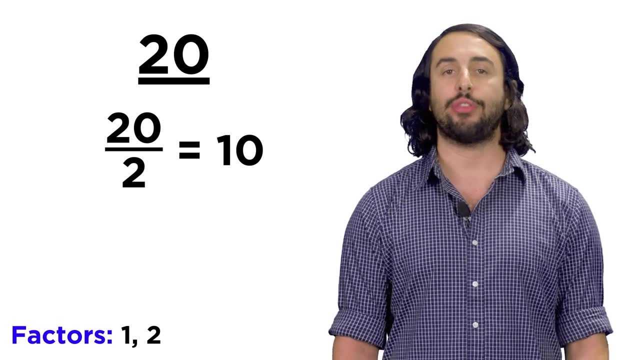 One, two, five and ten are the factors of ten. How about twenty For twenty? we see that one works, One works as always, Two as well, because it's an even number. Three does not, but four does as well as five. 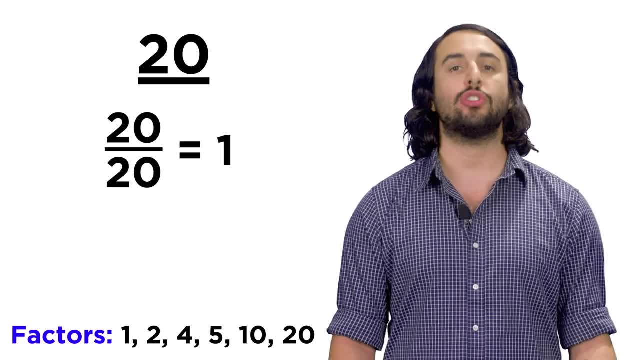 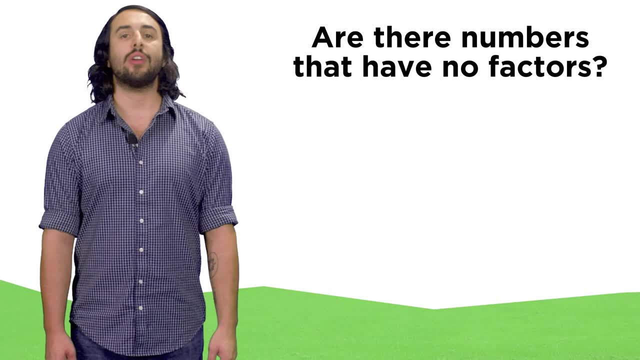 Then we jump all the way to ten, since it's half of twenty, Then twenty itself, and that's the end. Those are the factors of twenty. This brings us to an obvious question: Are there any numbers that have no factors whatsoever? 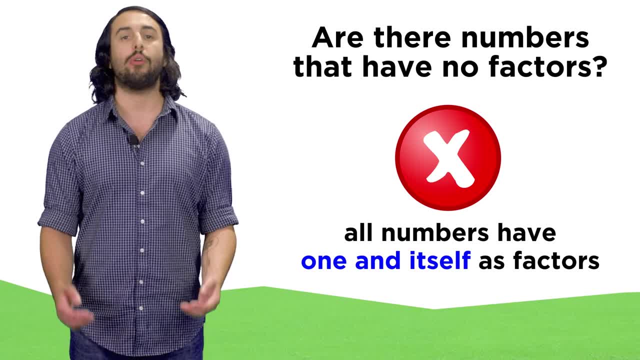 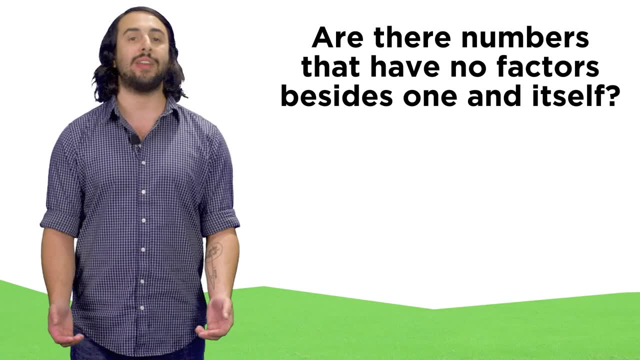 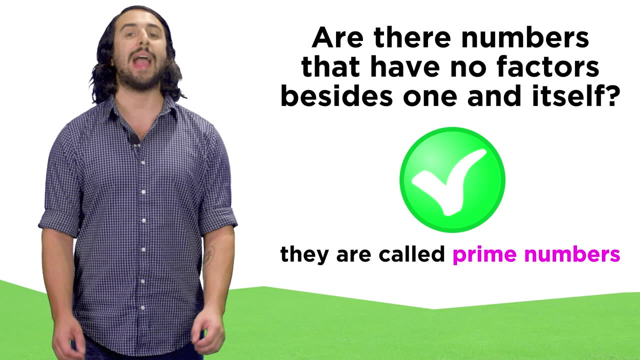 Technically no, because any number will have as factors both one and itself. But what about beyond that? Are there any numbers that have no factors besides one and itself? There are indeed many, and numbers that fulfill this criterion are called prime numbers. 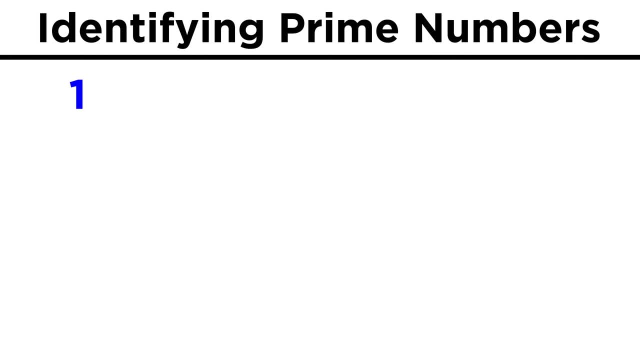 What are the prime numbers? One doesn't count, because one and itself would be the same thing. So let's start with two. Two counts, as does three, because these are so small that there can be no other factors. But once we get to four, four is divisible by two. 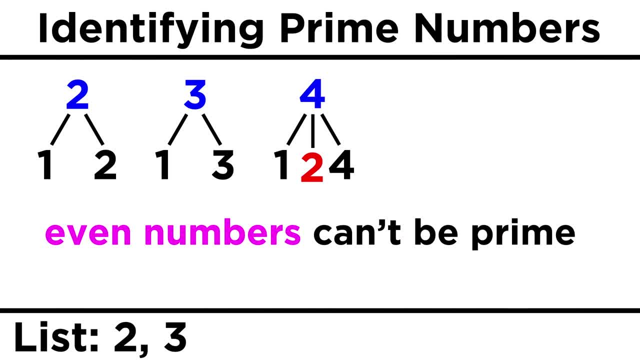 So four is not a prime number. In fact, no even numbers, except for two, can be prime numbers, because they are all divisible by two. Only odd numbers can be prime numbers. Five is a prime number, as is seven, but nine is not, because it is divisible by three. 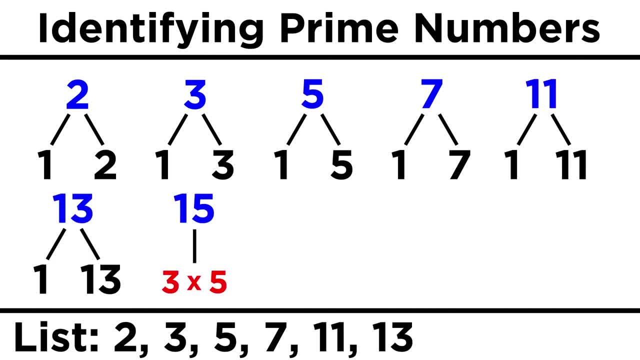 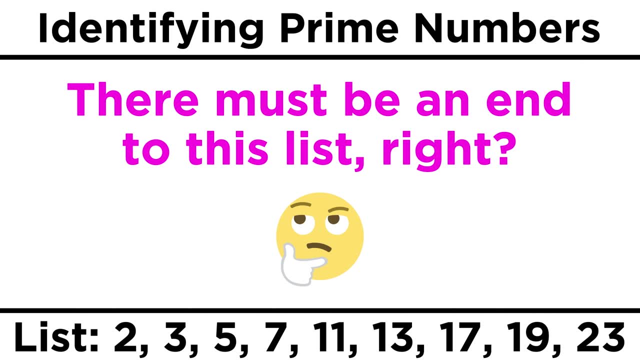 Eleven works, as does thirteen, but not fifteen, since that's the product of three and five. Seventeen works, and so does nineteen, but not twenty-one, since that's seven times three. Twenty-three works, and so on. One would think that this can't go very far, because once numbers get big enough, 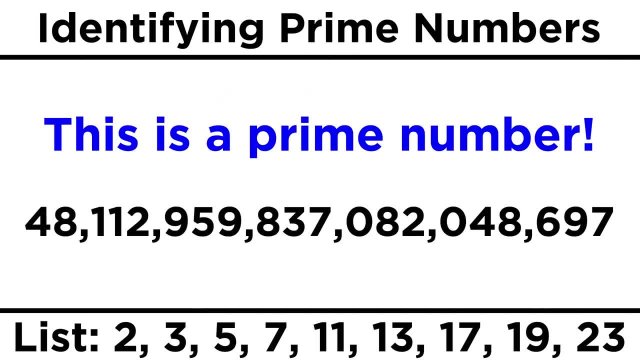 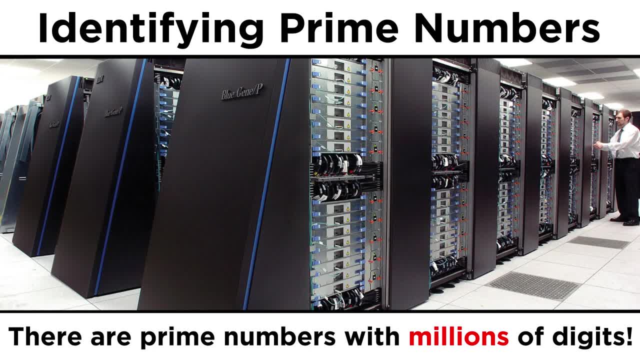 there have to be some factors in there, But there are some astoundingly huge prime numbers. The largest one discovered so far has millions of digits, which is mind-boggling, and it took thousands of computers running simultaneously for days to find this number. 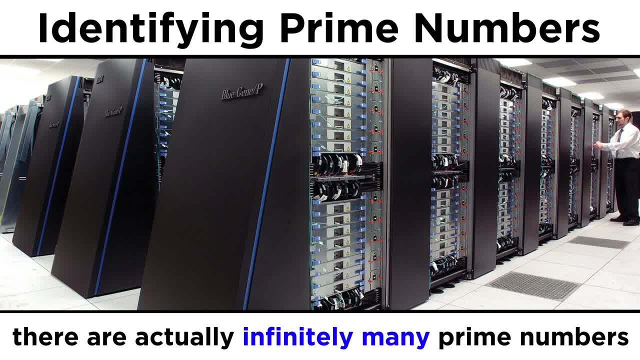 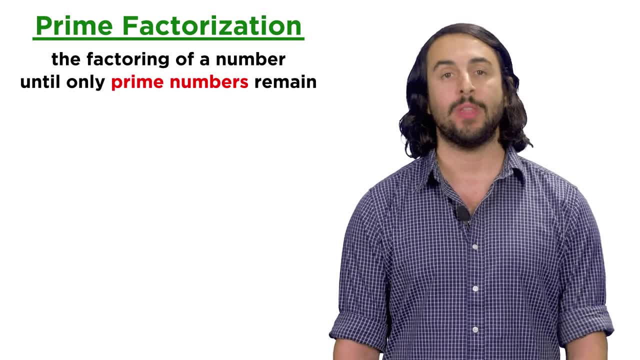 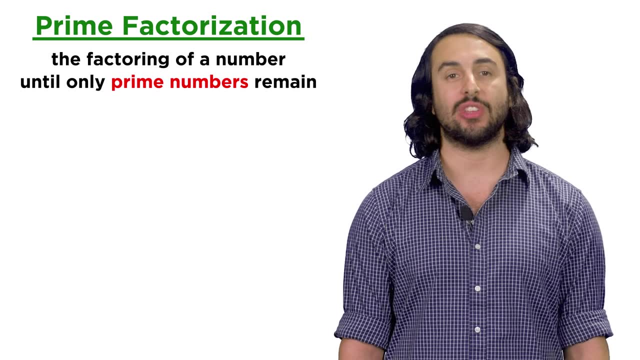 But there are infinitely many prime numbers, so no matter how big the biggest one we found, there's always a bigger one. So now that we know what prime numbers are, we can understand why we must factor numbers until only prime numbers remain, since that's the farthest we can go.